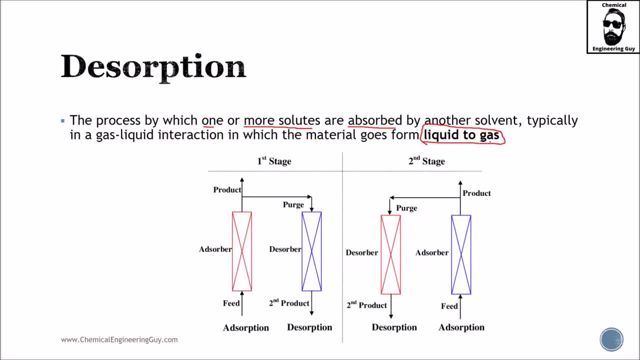 So here was gas to liquid. now it's liquid to gas. Why would you want to do that? Maybe because the liquid is more valuable for you, So I don't want to show you any complex materials. absorb it: desorber. 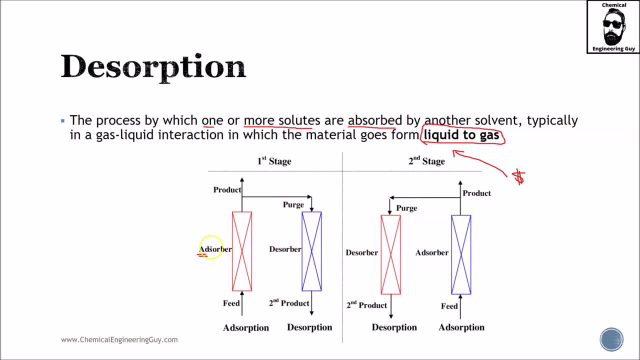 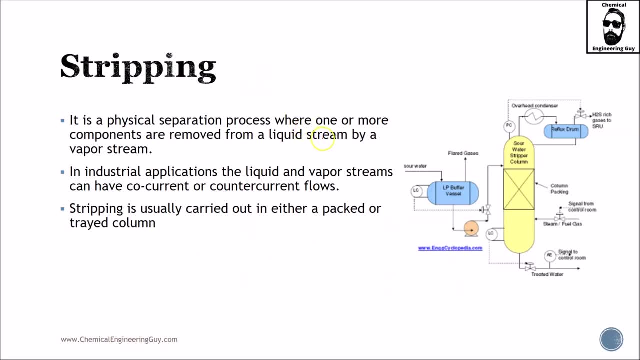 So, yeah, remember that this is not the same as absorption, But desorber is in fact what we're talking about. Stripping is pretty similar. It is a physical separation process where one or more components are removed from a liquid stream by a vapor stream. 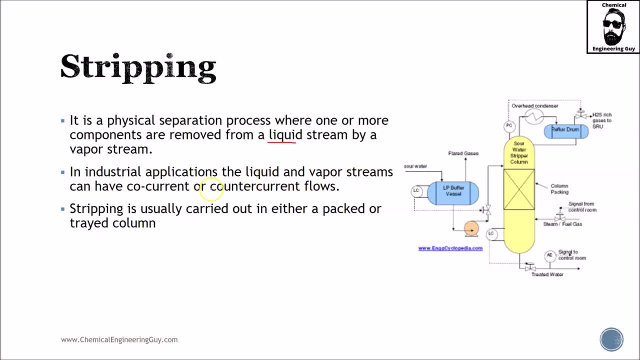 In industrial applications, the liquid and vapor streams can have co-current or counter-current flows. This is nothing more than. where are you going to feed the liquid? Is it going to be from the top or from the bottom? Stripping is usually carried out in either packed or tray columns. 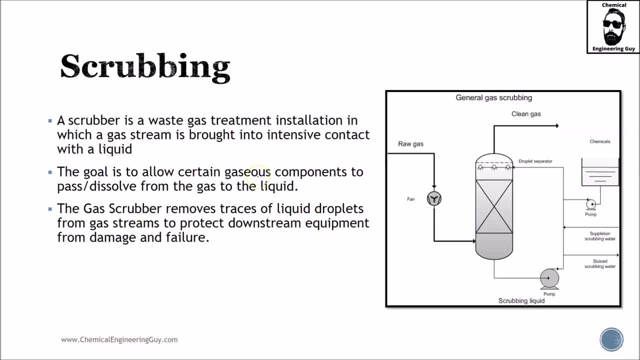 which we are going to cover in further courses. And then comes scrubbing. Maybe you have heard that before. Scrubber is essentially a unit operation which treats gases- waste gases technically- in which gas stream is brought into intensive contact with a liquid. 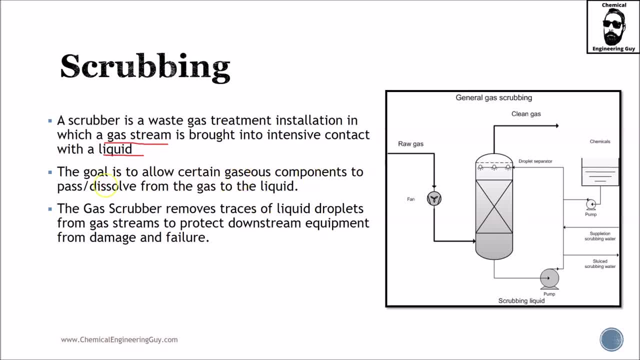 The goal is to allow certain gaseous components to pass or and dissolve from the gas to the liquid. The gas scrubber removes traces of liquid droplets from gas streams, which will further protect downstream equipment from damage and failure. Okay, well, as you can imagine, this is also a gas-liquid operation. 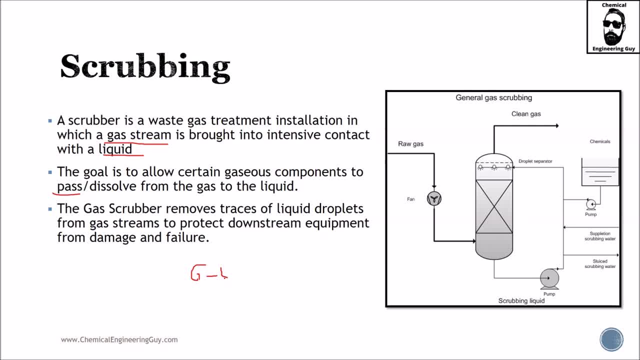 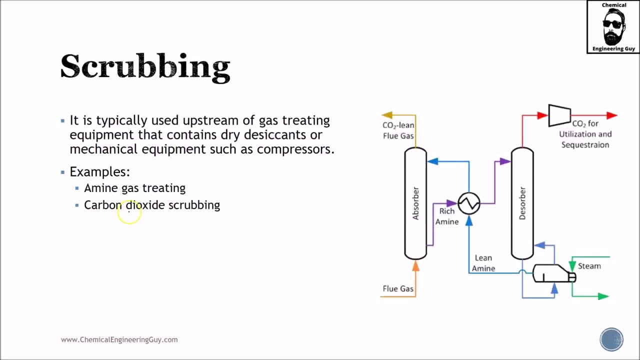 What we're doing here is cleaning our gas of interest with a solvent. Not only that, we are going to remove the droplets as well. It is typically used upstream, As you can see here, you have your gas going upwards and you have your liquid going downwards. 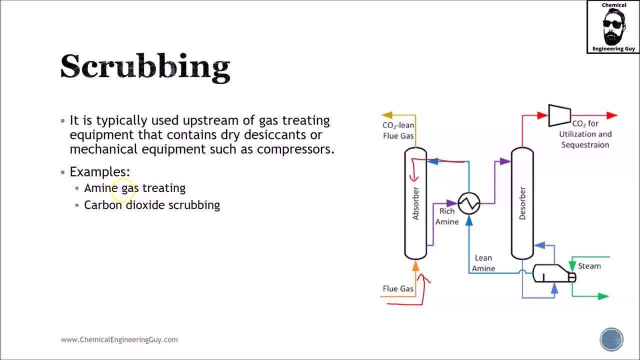 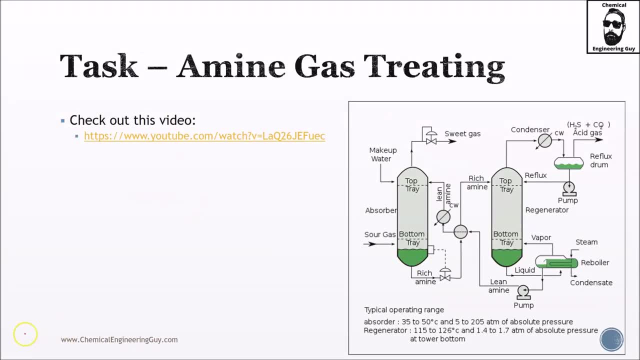 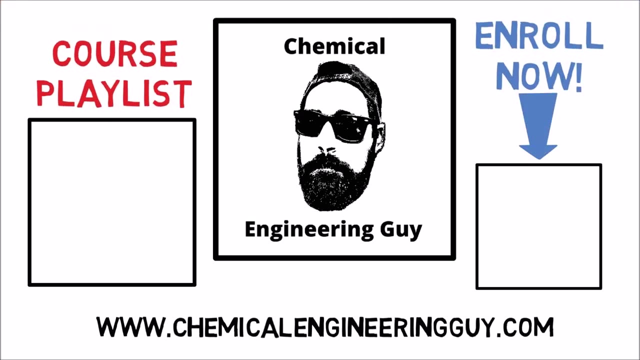 So it's countercurrent And the most common example will be amine gas treating or carbon dioxide scrubbing. Thank you,